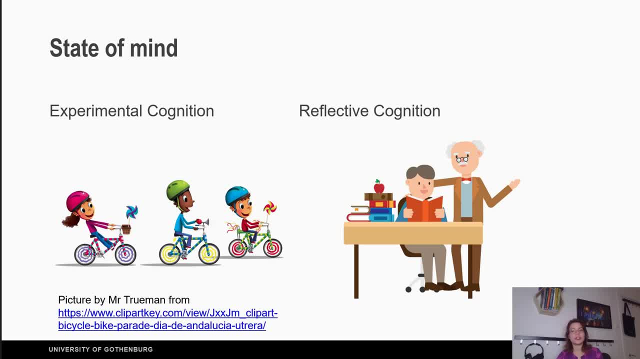 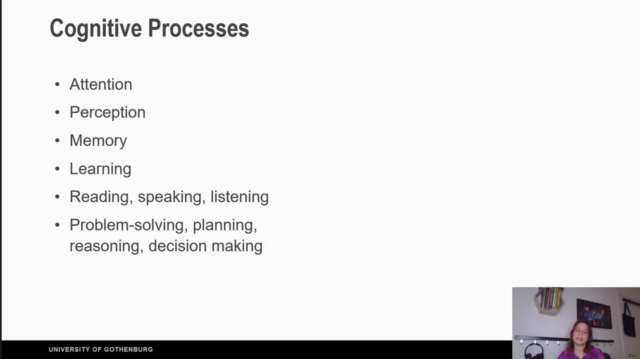 Experimental cognition is related to actions that we do and they need no or minimum mental effort, while reflective cognition is related to actions that they need more mental effort. Cognitive processes: In the book there are six categories of cognitive processes: Attention, perception, memory, learning. 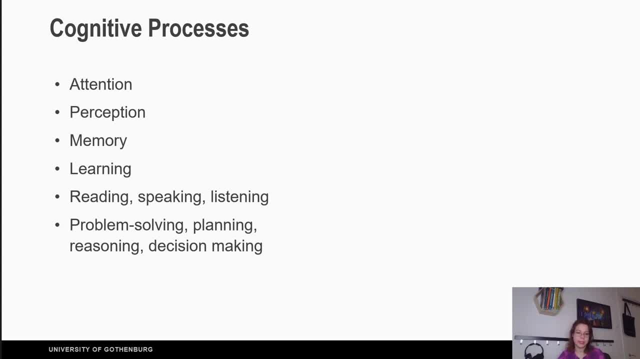 reading, speaking, listening and problem solving, planning, reasoning, decision making. Attention is related to our focus on tasks. We can focus only on one task and we cannot split our attention. The word multitasking doesn't mean that we pay attention to do different things. It actually means that we can change our attention. 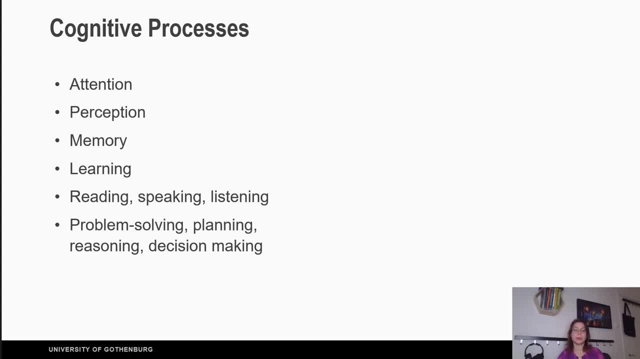 to different tasks, and other people may think that we pay attention to do two different things. Perception is the understanding of the world based on our senses and cognition. We have two types of memory: The short-term memory and the long-term memory. In the short-term memory we store information that we just listen. They don't stay in this memory for. 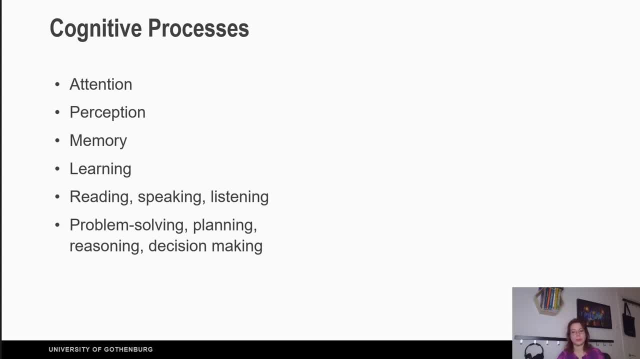 long. Either we forget them or they move to the long-term memory. In the long-term memory, we store information for longer time. Learning Learning is the process that transfer information from the short-term memory to the long-term memory. Reading, speaking and listening are 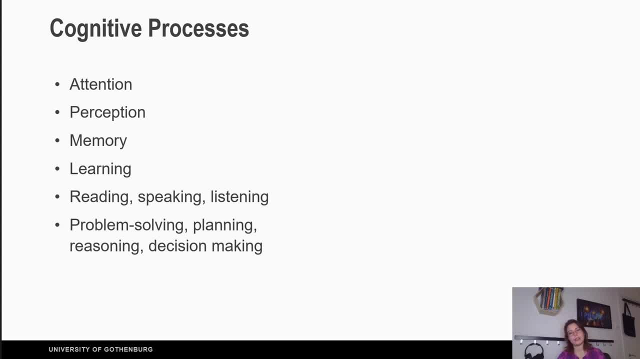 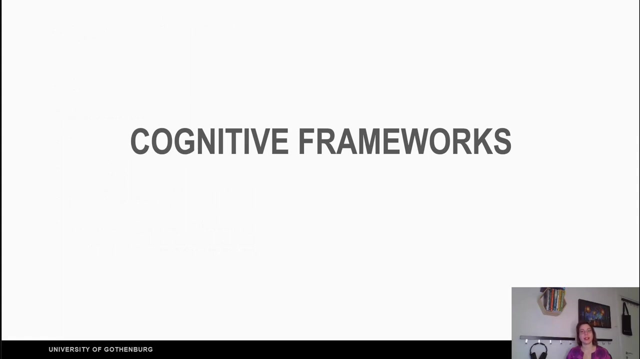 related to the language processing skills and they vary from person to person. For example, people with dyslexia may have difficulties on reading. Finally, problem solving, planning and reasoning are processes that involve reflective cognition, Cognitive frameworks. Cognitive frameworks help us understand and predict user actions in relation to our interface. 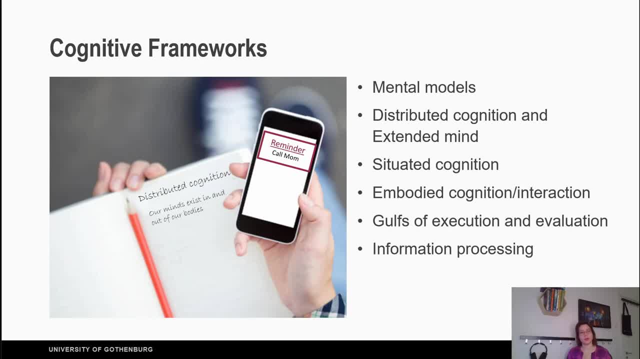 There are several cognitive frameworks. One of them is mental models. Mental model is the model the user builds in their mind for our interface. For example, when it comes to Microsoft Office, if you have used one of them, like Word, you will easily be able to use PowerPoint or Excel, and you will find. 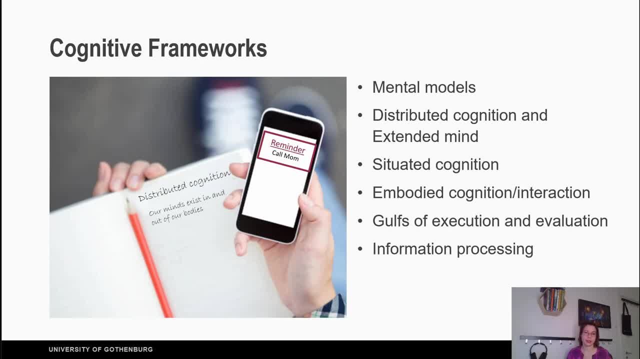 the common functions because they are all in the same place, and you have built already a model on how, for example, can someone copy paste text in the Microsoft products Distributed cognition and supports that the mind is extended, That the mind doesn't exist only inside our head, but it is extended to different. 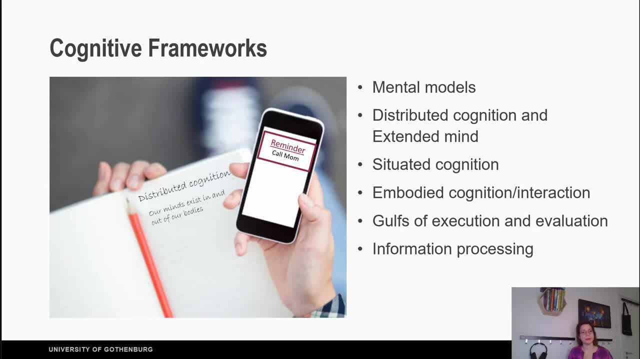 artifacts and other people. For example, as we see in the picture, distributed cognition thinks supports that. the reminder on our cell phone is part of our cognition. A better example is an airplane cockpit where the pilot and the co-pilot reduce our comprehension of theuh. co-pilot of the flight. 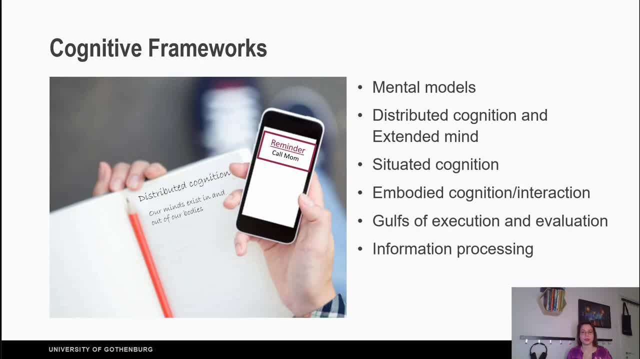 And we also see that the AI Mustang uh using a loss on the entire team. The problem is the fact that the AI mankind is so complex and its our mind is completely created from our own account, uh, sort of. and it's not. it's not yet. 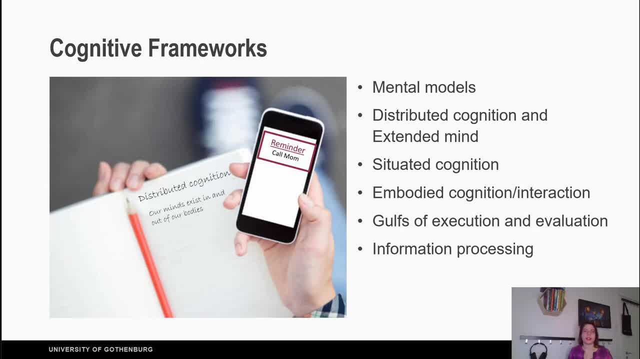 an environment that we can create. So it's okay to be uh uh, be a pounds in a to uh uh in this world, um uh. in this world of us, um uh. in this world of minds, um and um, uh uh. 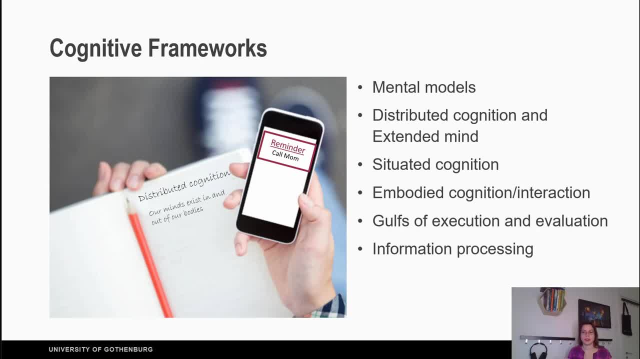 The space and the around, the um uh, um, uh, um, uh, um, um, um, oh. yeah, we assume that the mind is shaped based on our bodily interactions with the environment. The gulf of execution and evaluation is the mismatch.